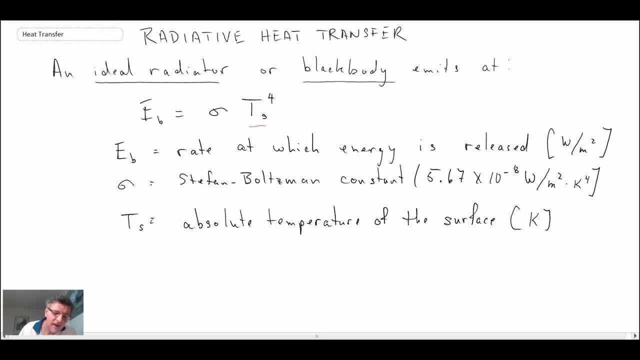 particular temperature, and the temperature of the body would be ts, and the proportionality constant in this equation is the stefan boltzmann constant. now, one thing that i should say that you have to be very, very careful of when you're using these equations, and radiative heat transfer is notice. 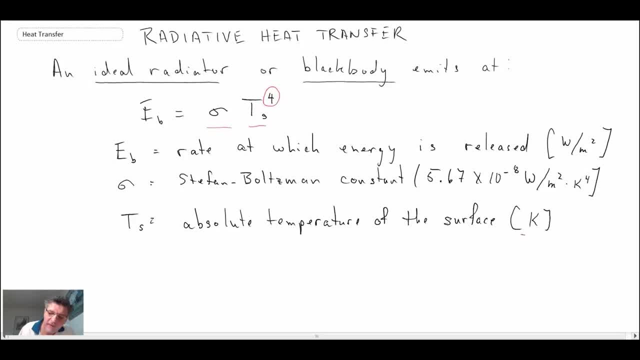 we have this raised to the power four, and so therefore you need to ensure that your temperature is always in kelvin. if you try putting degrees celsius in here, you will get the incorrect value, so be very careful with that. now, an ideal radiator. that's kind of a theoretical maximum, that an 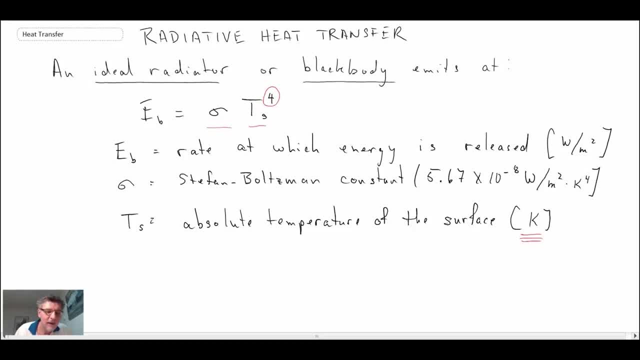 object would emit at a given temperature. in reality, no objects emit at an ideal radiator. they emit at a slightly lower value than that, and in order to characterize that, we have a term called the emissivity. so let me show you the equation for how a real object would respond. 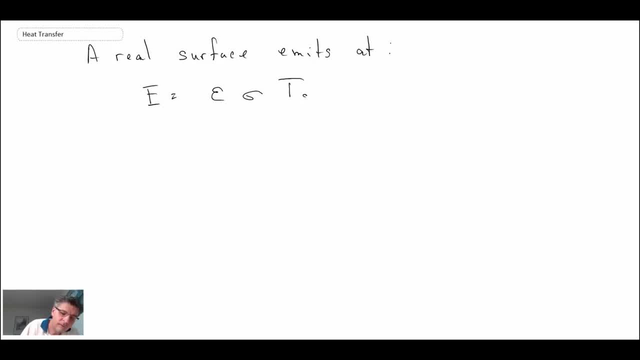 and so that would be a real surface in comparison to a black body. notice, when we had black body, we had the b subscript. here we do not have it for the rate at which energy is released, the term on the left hand side, and we also have this new term that we've introduced, this epsilon. this is the emissivity. 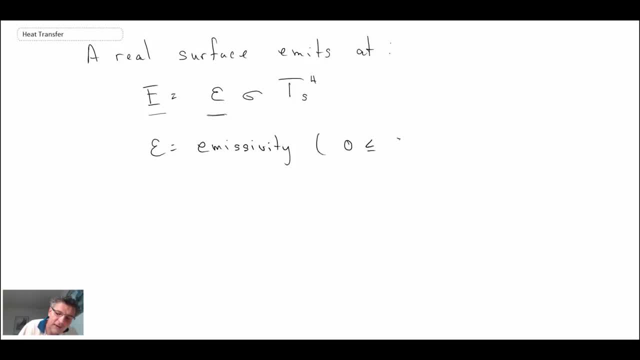 and the emissivity is going to range between zero and one and depending upon the object that you're doing the calculation for looking at. there are tables with emissivities and surface finish is very important for emissivity, be it dull or very, very polished. that can have a big impact on the 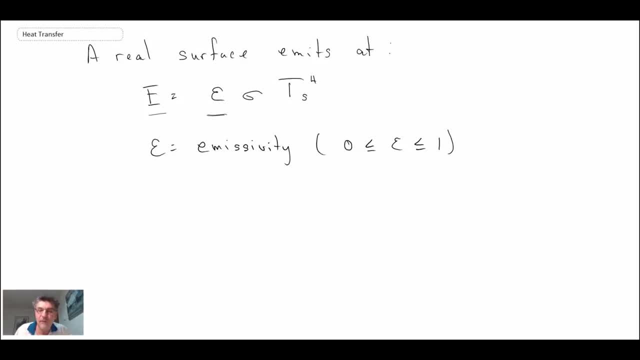 emissivity, so that is in terms of what an object would emit. we're all radiating energy right now- radiative heat transfer- so that's going to be a very important part of the calculation for looking at, and the emissivity is going to range between zero and one and depending upon the object that you're. 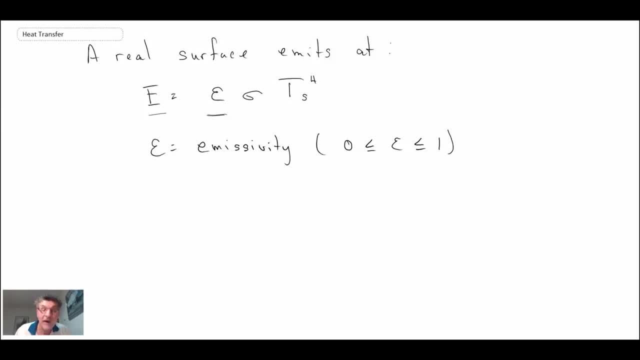 doing the calculation for looking at. there are tables with emissivity, and surface finish is very important for looking at heat transfer, given the temperature of our bodies versus the surroundings. at the same time, the surroundings around us are radiating and we're absorbing the radiation from the surroundings and 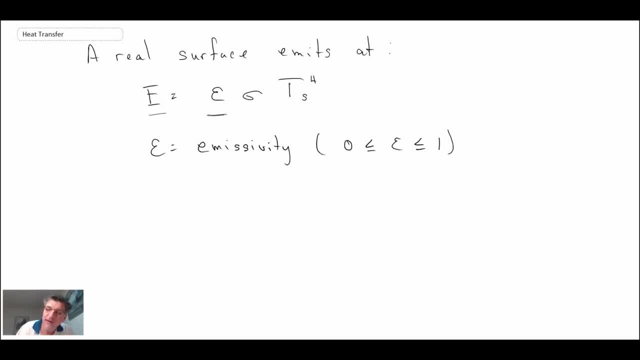 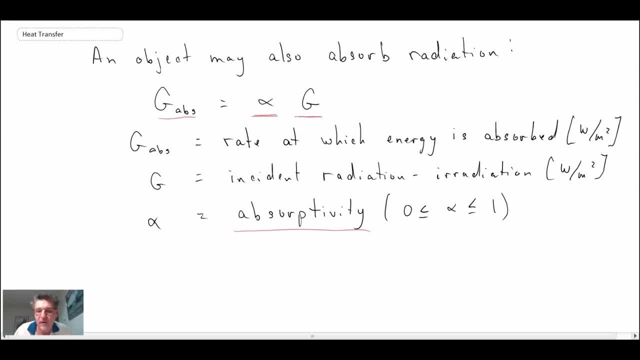 this term here. this is the incident: radiation, sometimes called the irradiation, and that would be the amount of radiative energy coming onto a particular object and- and so a very simplified case of this- we we could look at a smaller area versus a larger surrounding, so let's take a look at that. 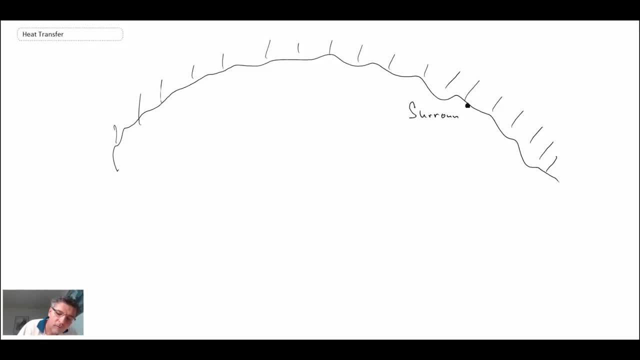 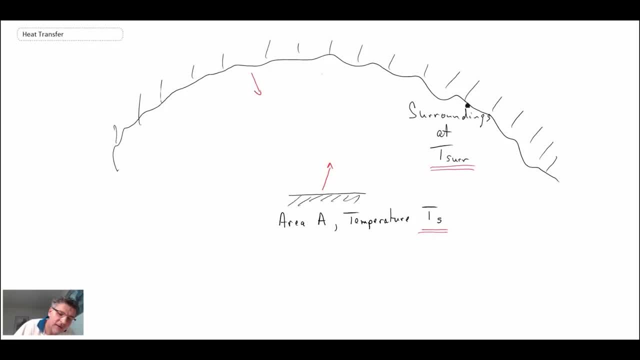 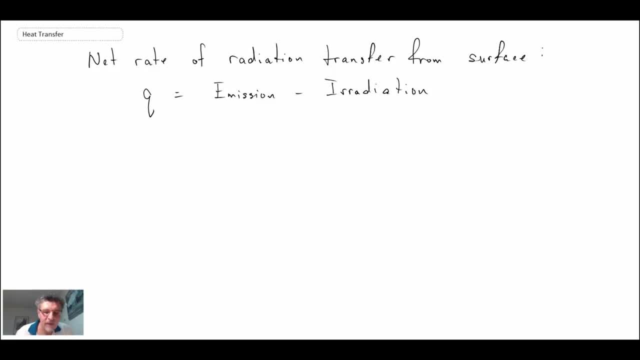 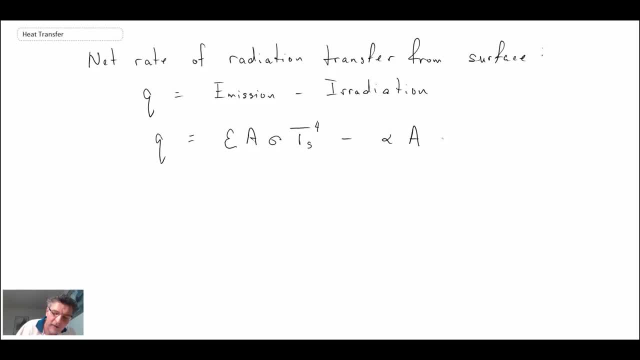